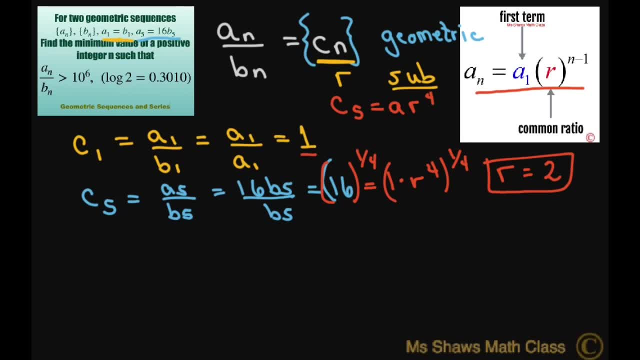 that we have our common ratio and our first term. we can write our formula: C sub n equals 1 times 2 to the power of n minus 1, again using this formula: okay, okay. so now we know that a sub n divided by B sub n is greater than 10 to the power of 6, so that 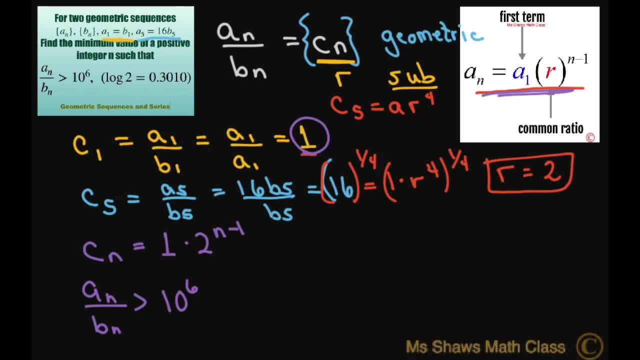 means. let's see: C sub n is greater than 10 to the power of 6, which means 2 to the power of n, minus 1 is greater than 10 to the power of 6. now we need to solve for end. so that's what we're looking for in. so let's do that and write this: 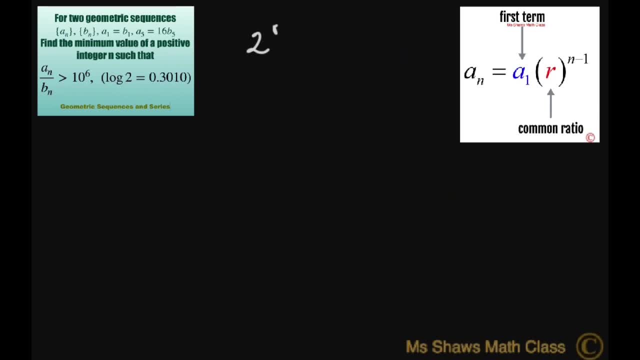 again we have a 2 to the power of n minus 1 is greater than 10 to the power of 6. so I'm going to do is take logs of both sides, get this in out of the exponent. all right, using your power property, let's move this power down. so. 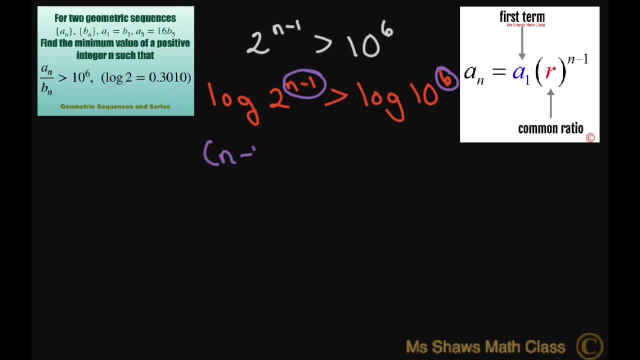 we're going to get in minus 1 times log of 2 is greater than 6 times log of 10. now, since there's no base written here, this is log base 10 of 10 and this equals 1. so basically what we have is n minus 1 times log of 2 is greater than 6. this is: 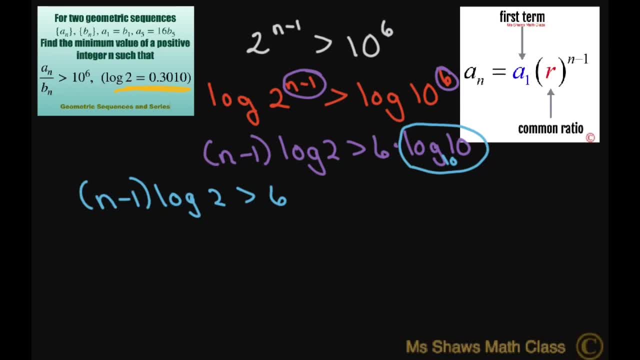 where this comes in, so we can substitute this in. I'm going to write this as: n minus 1 is greater than 6.. I'm just dividing by log of 2.. But log of 2 is this number here, So I'm just going to write this as 0.3010. 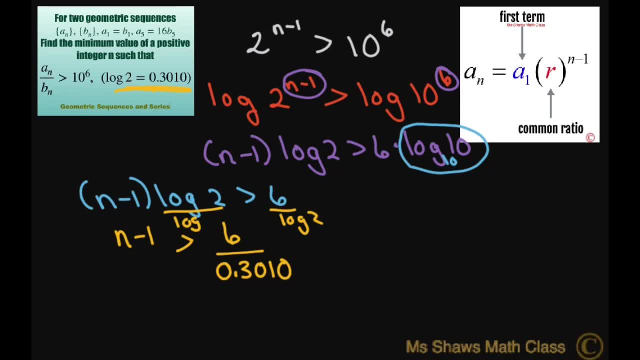 All right, That means we have: n is greater than 6 divided by 0.03010.. And we have to add 1.. All right, When you get that, you're going to get n is greater. This is going to equal 19.93 plus 1..